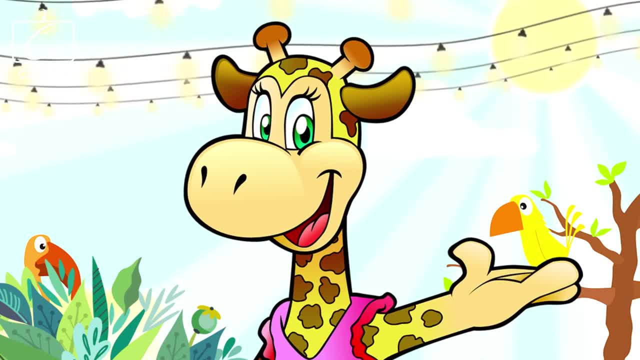 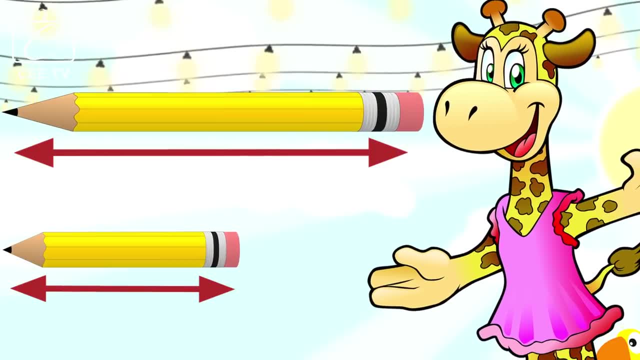 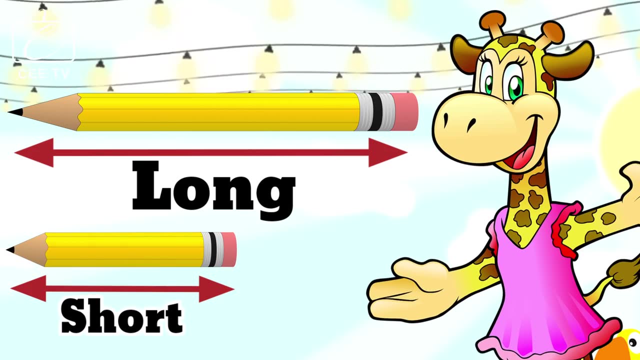 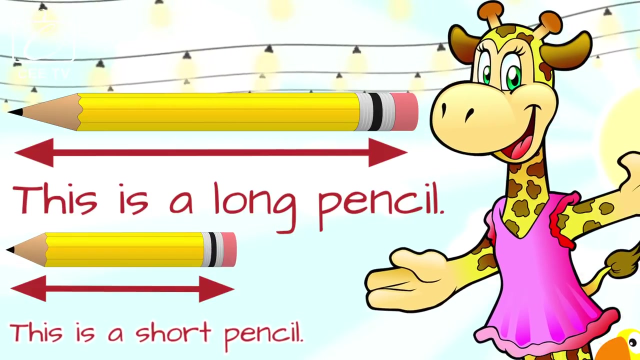 Hi kids. Today we are going to identify and compare lengths of objects. Objects have different lengths. Some are long and some are short. This is a long pencil. This is a short pencil. We use the words long and short to describe length. 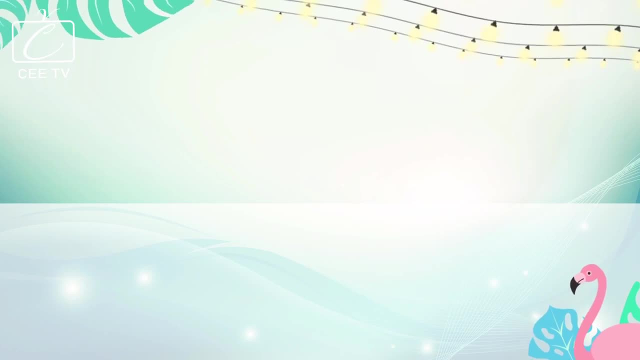 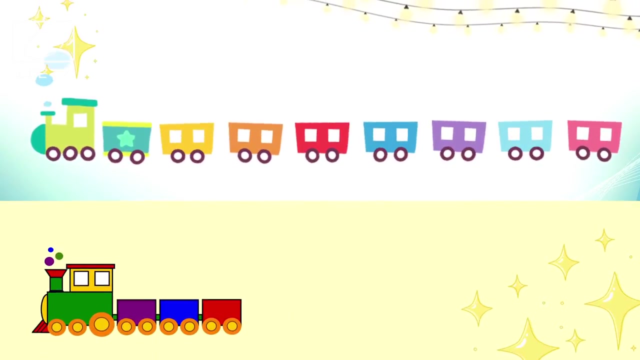 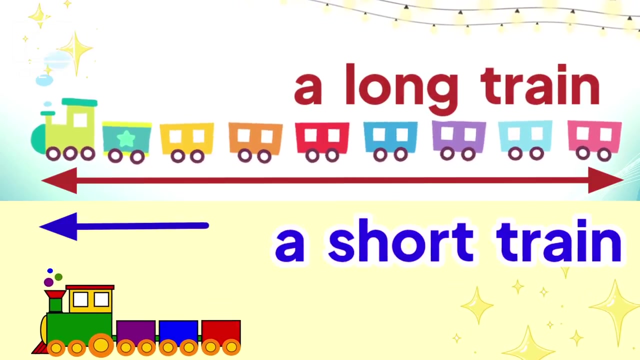 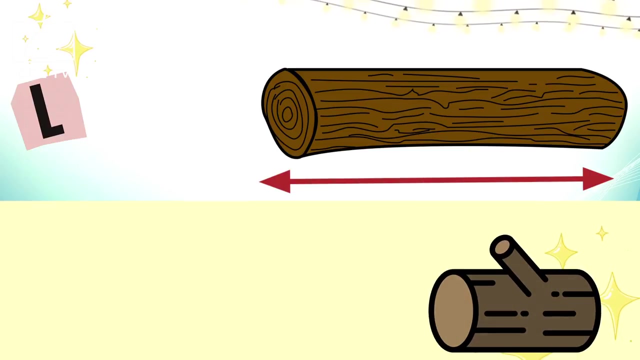 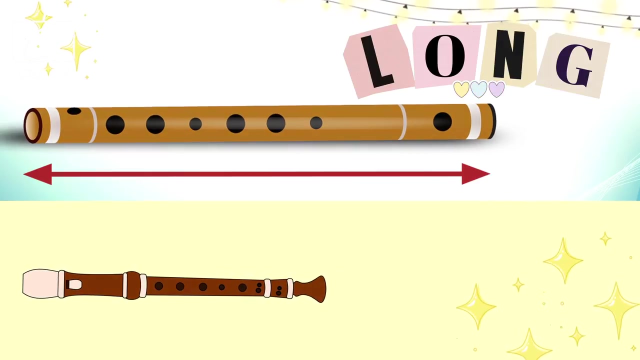 See TV: Long Short, Long Short, A long train, A short train, A long train, A long train. Long Short, A long log, A short log, A long log, A long log. Long Short, A long flute, A long flute. 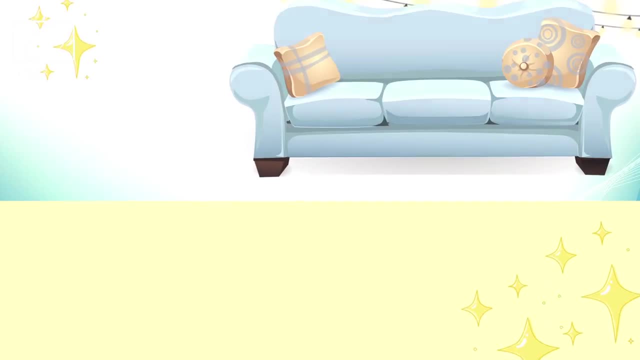 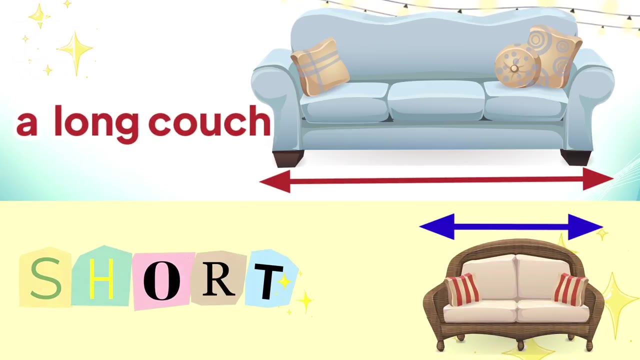 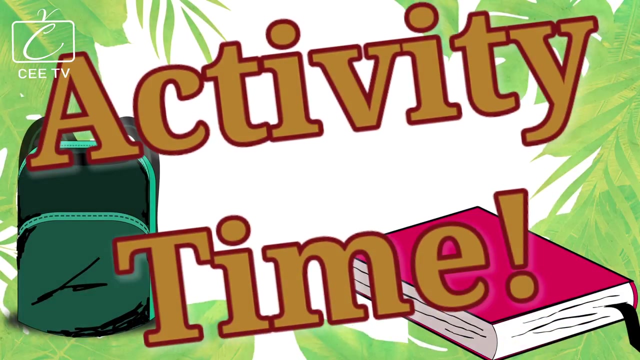 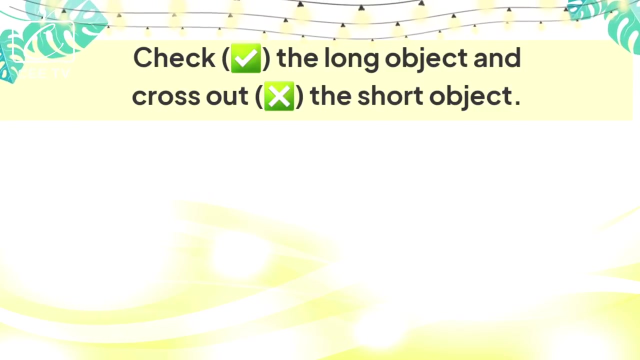 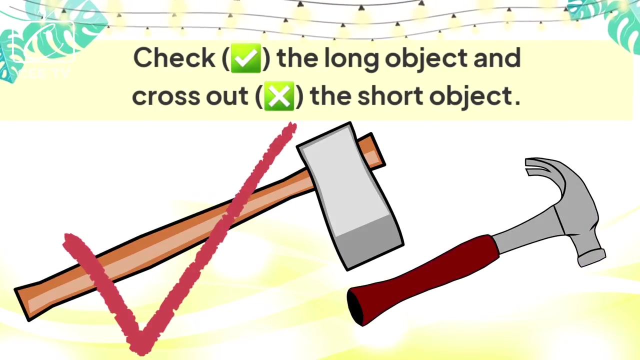 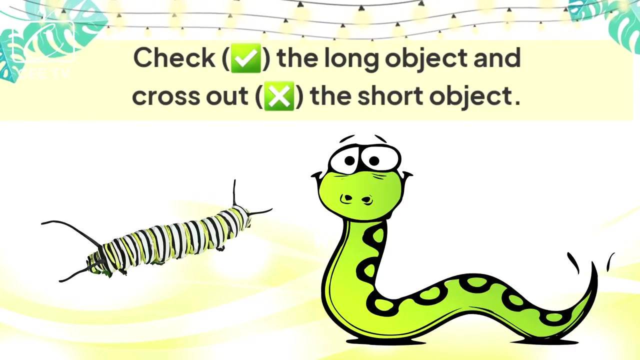 A short flute, A short flute. Long Short: A long couch, A short couch. Activity time: Check the long object and cross out the short object. The axe is long and the hammer is short. The caterpillar is short and the snake is long. 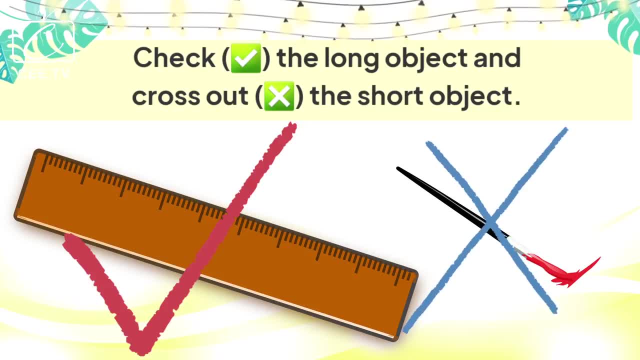 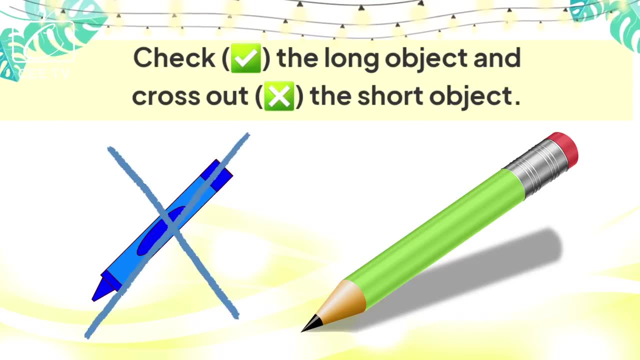 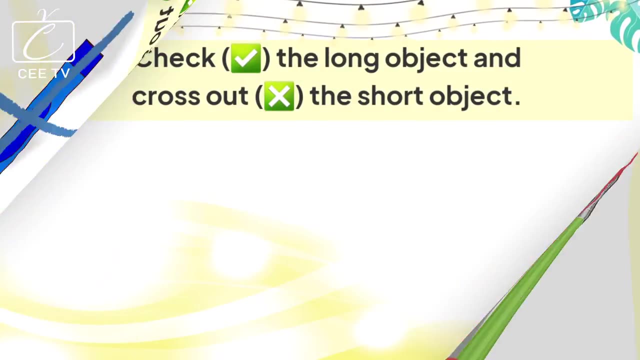 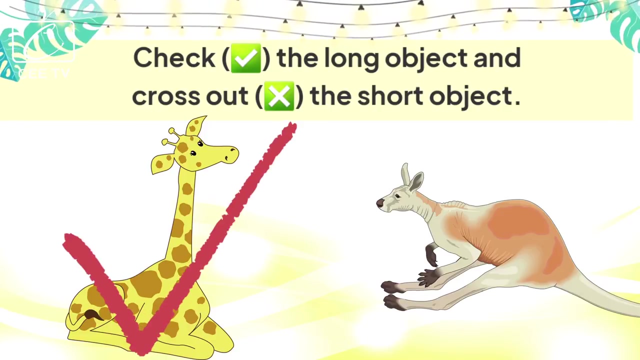 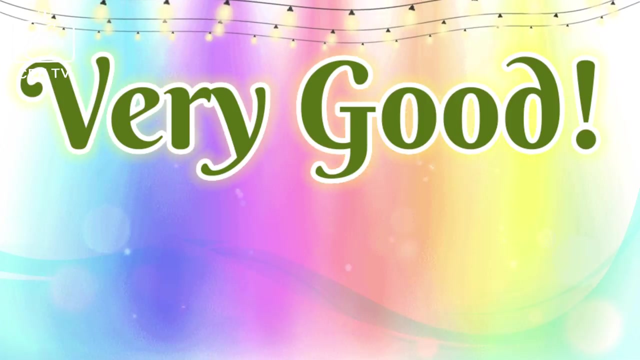 The ruler is long and the paintbrush is short. The crayon is short And the pencil is long. The giraffe's neck is long and the kangaroo's neck is short. Very good, You were able to identify the long and short objects correctly.